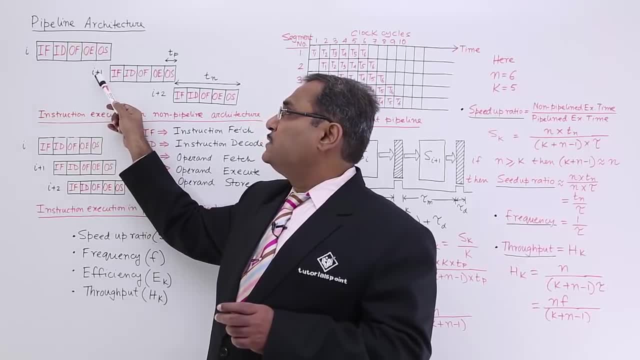 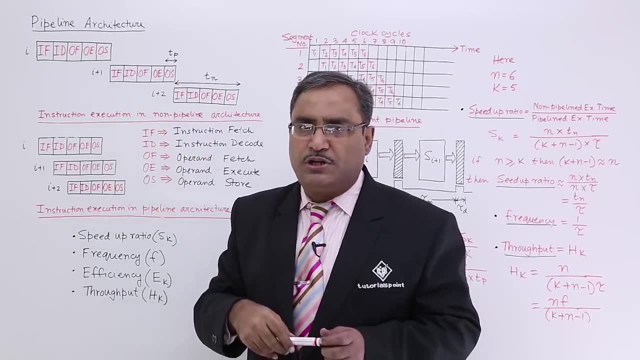 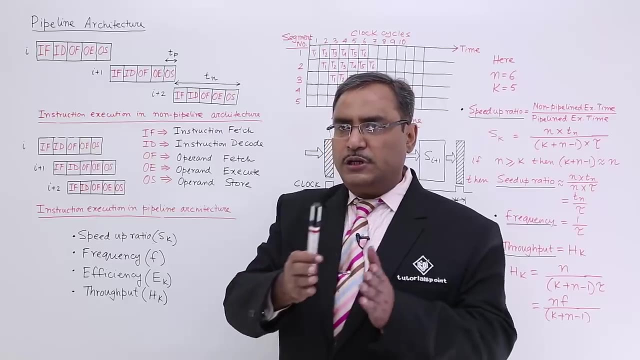 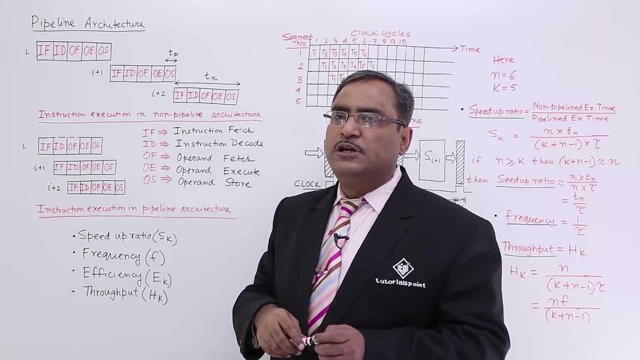 execution for the ith instruction, then i plus 1th instruction will be initiated. After completion of execution of i plus 1th instruction, then i plus 2th instruction will be executed. So instructions will go on executing After completion of the prior one. So they are executing and in a fashion known as instruction. 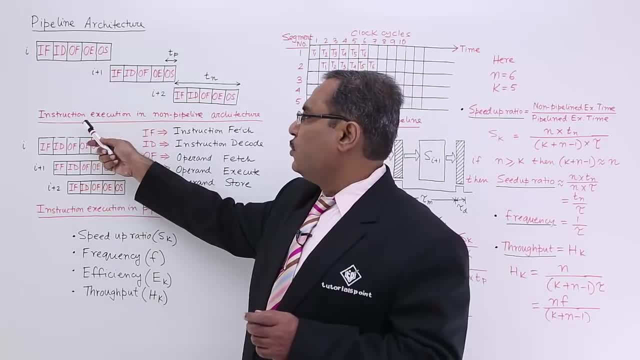 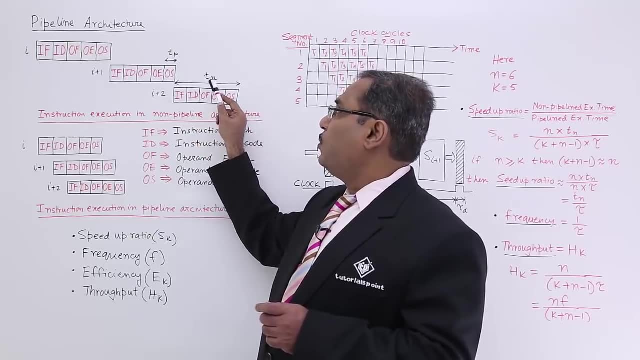 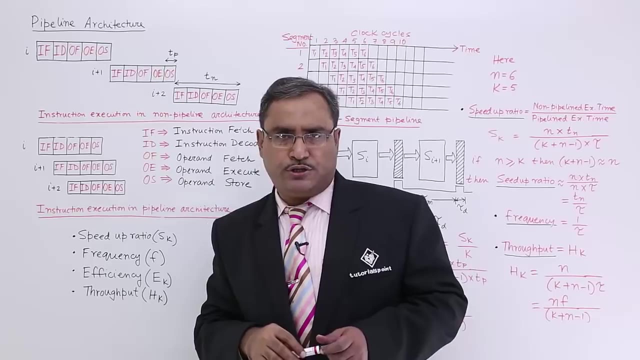 wise interleaved, So that is known as the non-pipelined architecture. Here this total instruction duration, execution duration- i can call it as tn and the phase duration i can call it as a tp. So tp stands for the phase duration. ok, In case of pipeline. 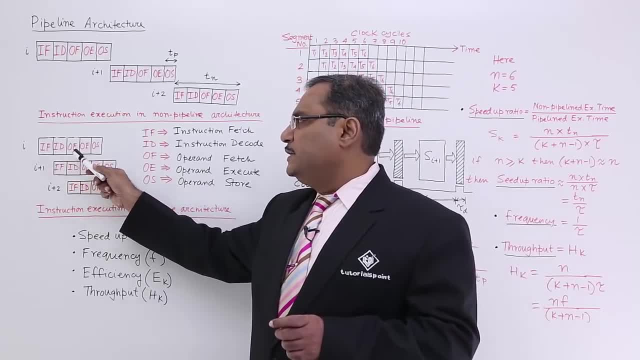 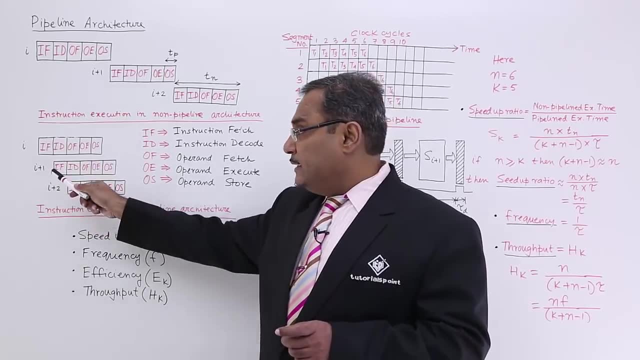 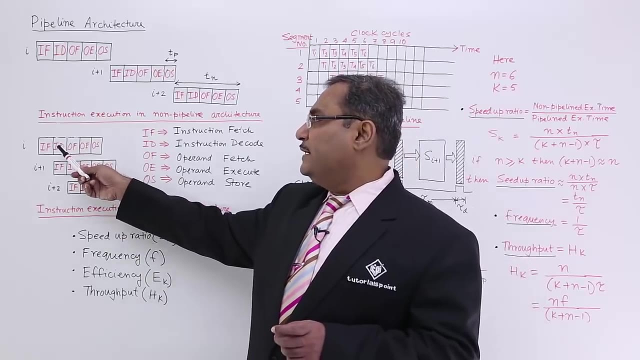 architecture: when the first instruction is executing, when the first instruction is going from first face to the second face, then the next instruction, that is I plus 1th instruction, will be going to the instruction fetch, And when the Ith instruction will be going. 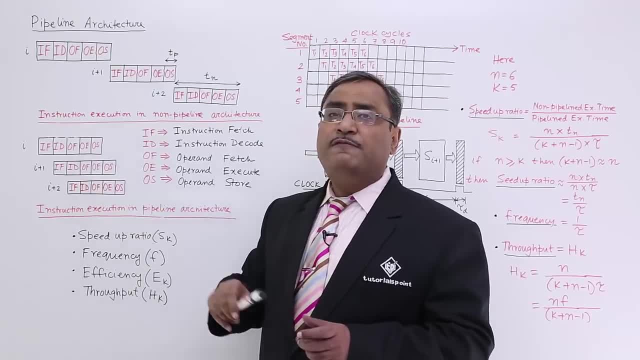 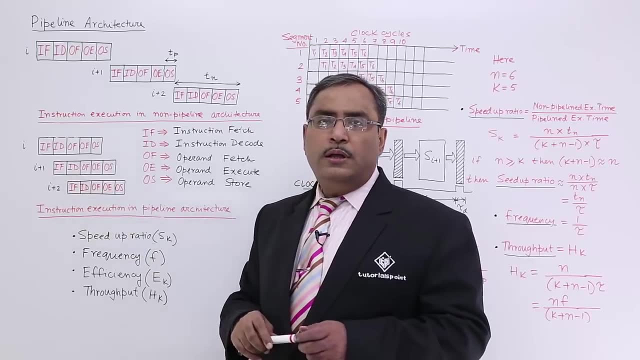 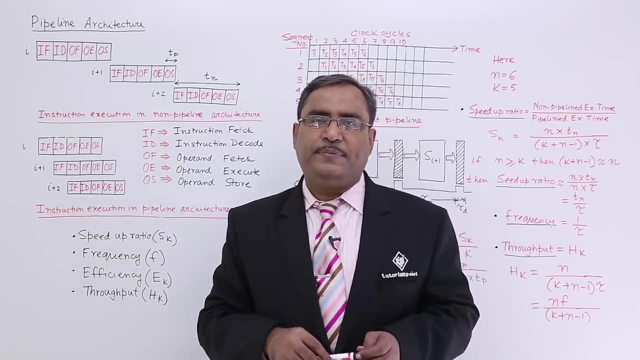 from the instruction decode to operand fetch face. then I plus 1th instruction will be going from instruction fetch to instruction decode and I plus 2th instruction will go for instruction fetch execution for the first time. So here this: instructions are getting executed, phase. 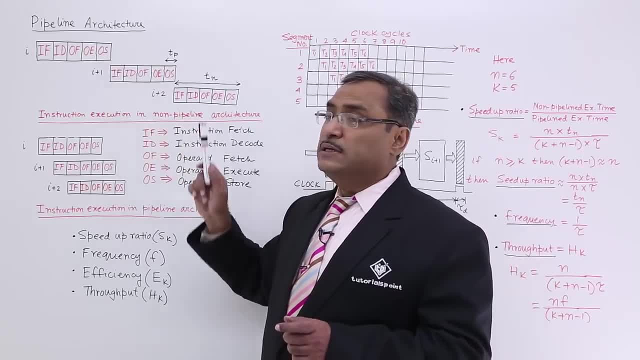 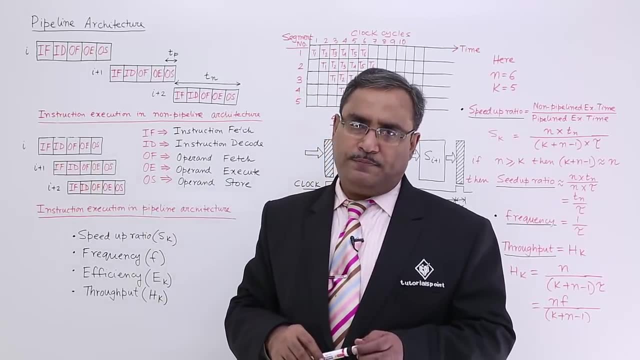 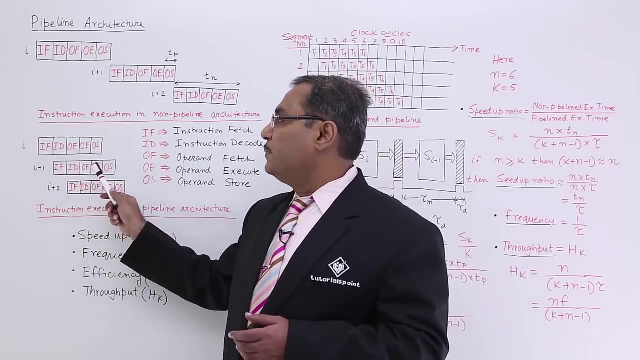 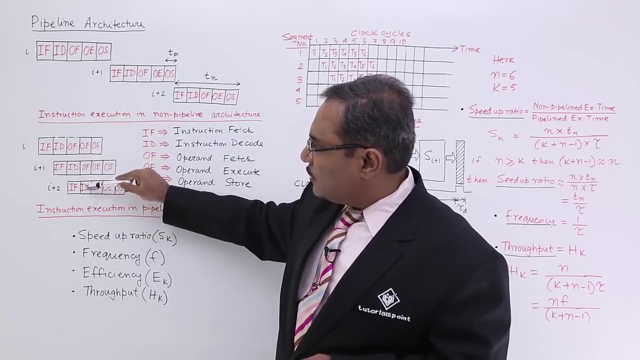 wise interleaved, whereas here it was instruction wise interleaved, So this is known as pipeline execution. here instruction execution time spans are overlapping, So parallel execution of instructions are taking place. if you consider any, just vertical, this one, just consider this particular time slot, you cannot find more than one instruction in the same phase. all. 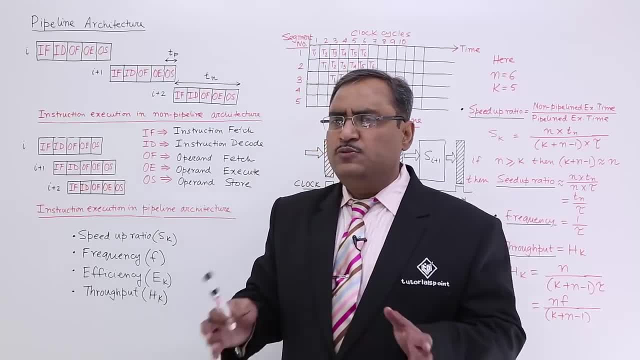 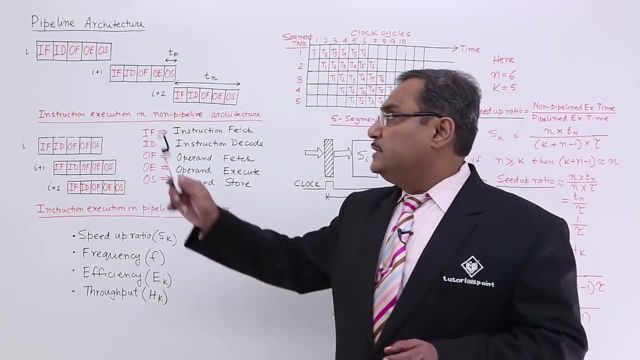 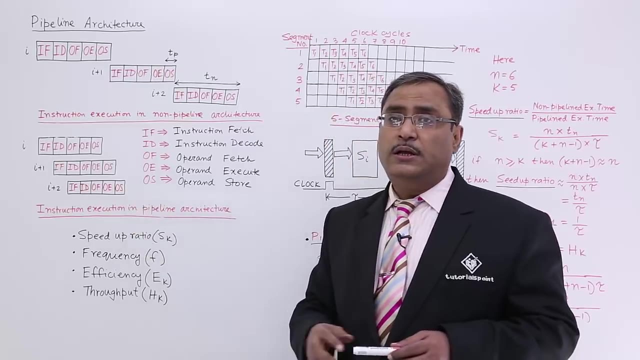 the instructions will be in different phases, So, phase wise, there will be no contention. So this is known as pipeline execution, This is known as non-pipeline execution. So obviously we can feel that in case of pipeline execution, the instruction will get executed or the program will get executed. 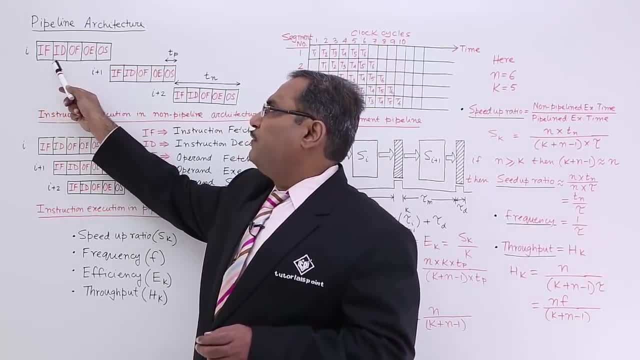 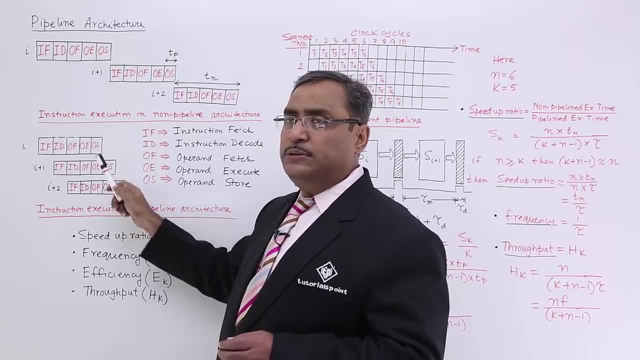 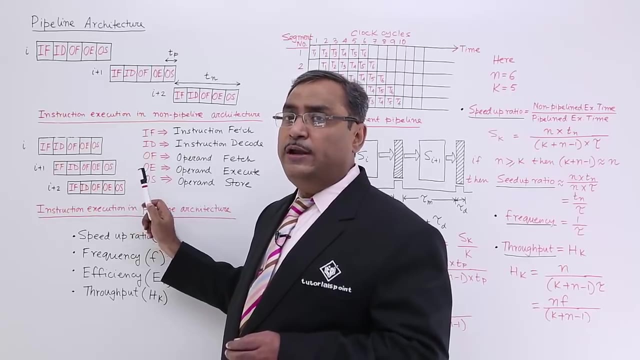 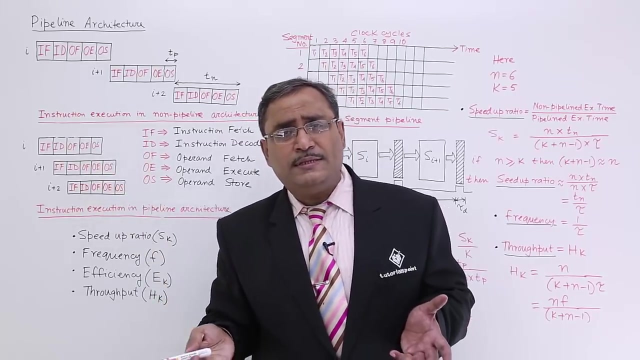 faster. How many cycles it took: 5 cycles into 3.. So 15 cycles, 15 phase durations it took. but here, to execute the same number of instructions, same number of 3 instructions, how many phase durations were required? 1, 2, 3, 4, 5, 6, 7, only 7, only 7 has suffice, this particular requirement. 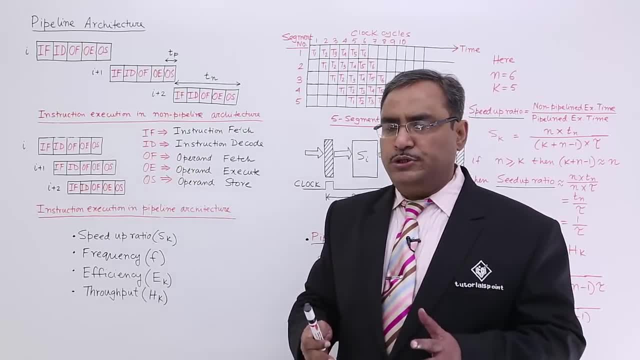 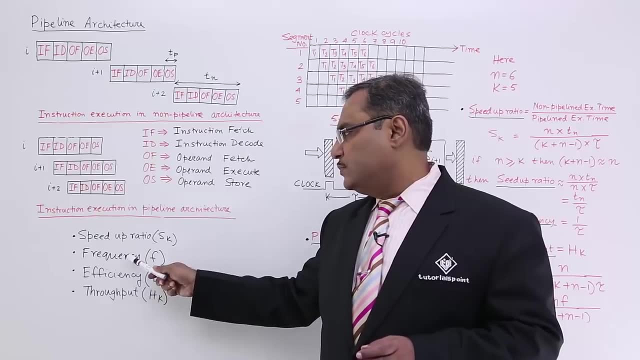 Now we shall discuss some parameters which will decide that how. what is the performance of your pipeline execution? So we shall discuss this. 4 parameters: one is the speed of ratio. next one is a frequency: how to calculate the frequency? next one is a pipeline efficiency. 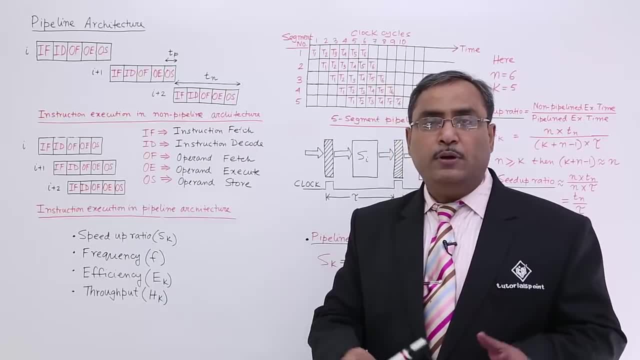 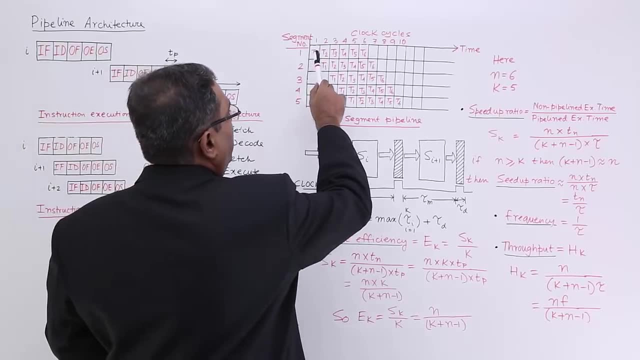 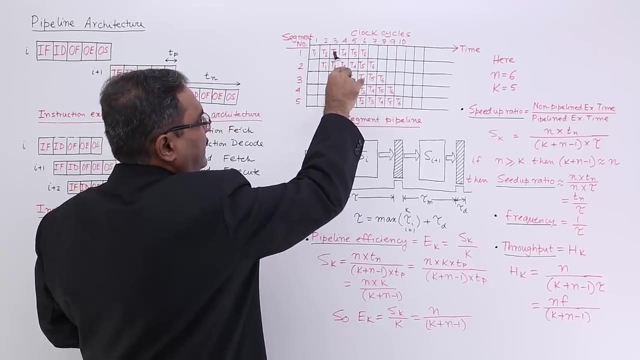 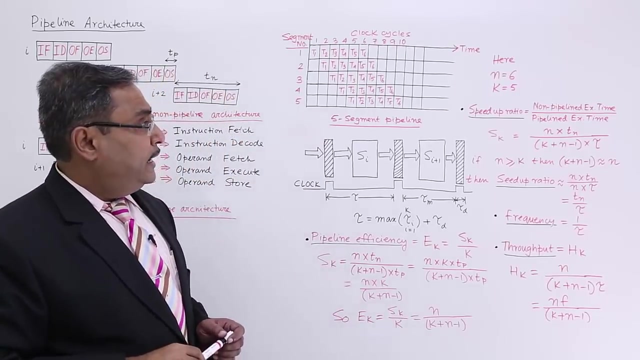 and the is a pipeline throughput. so let me go one by one. so i've done the board work here. let us suppose we're having five phases. this is the instruction number one. executing instruction number two. executing instruction number three. instruction number four, instruction number five, instruction number six. so here you see, at any duration of time you can find, find multiple instructions. 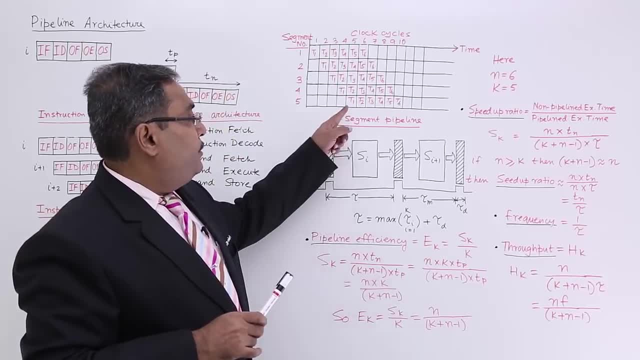 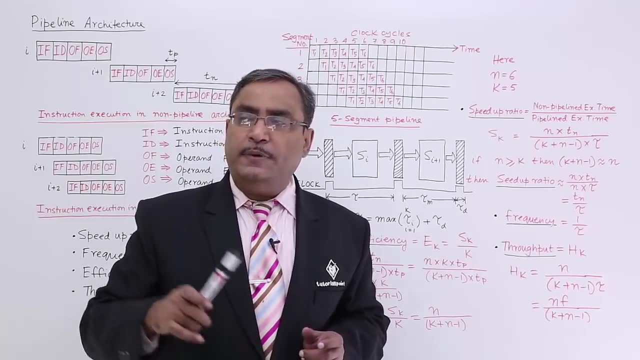 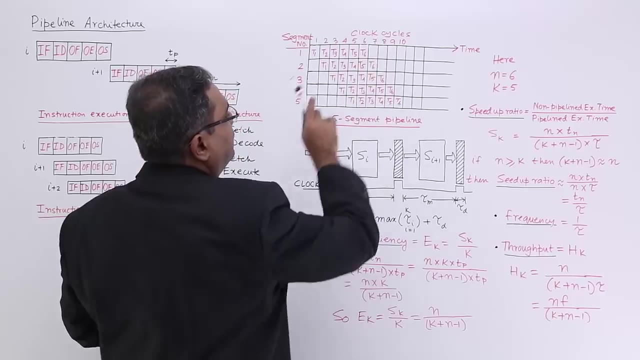 are working or executing at the same time, but you cannot find that in the same phase. multiple instructions are there. phase wise, they are interleaved, as i discussed here earlier. so that is the issue. so how many clock cycles did it require? how many, i'm telling you, here is five. 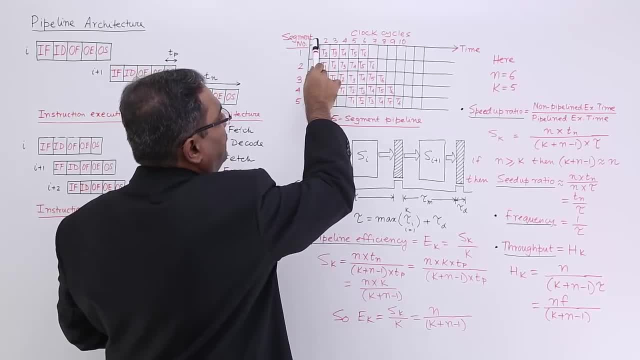 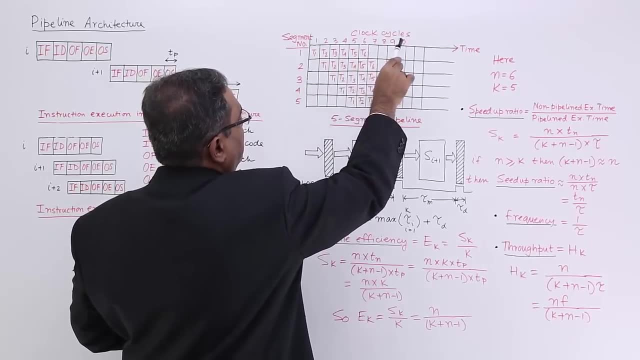 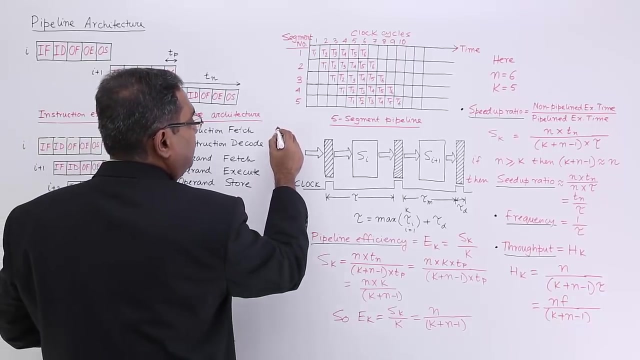 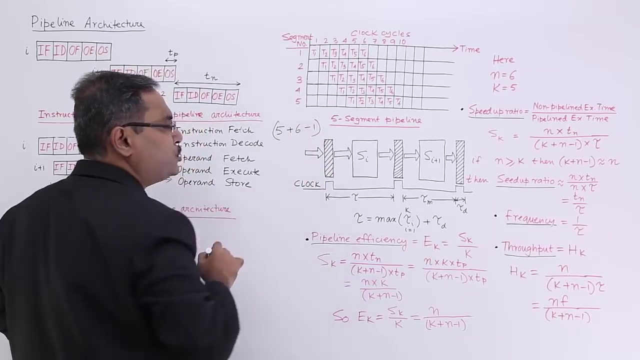 phases. are there segment or phases? so here we are having, uh, six instructions. are there t1 to t6? six instructions. so how many clock cycles it take, or say durations, phase duration it take, it takes 10 such. so i'm giving you five, i'm giving you six. so how to get 10? so the equation is n number of instructions. 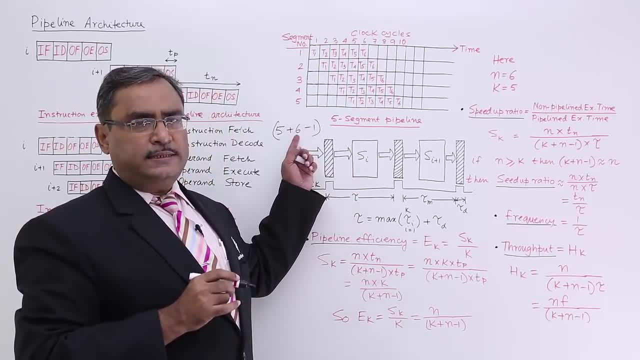 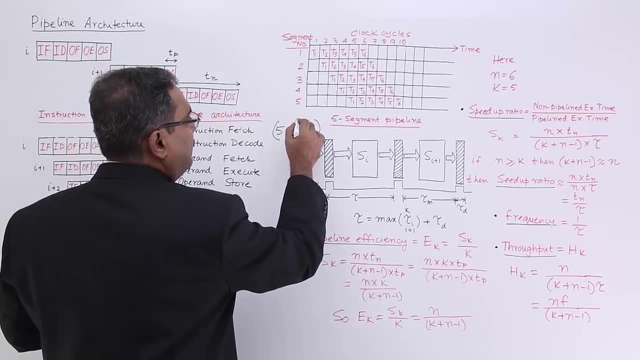 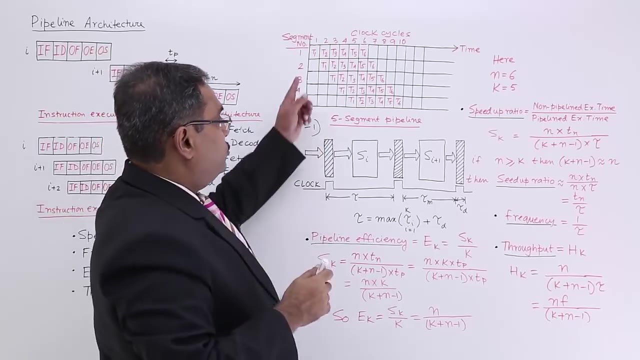 here the value of n is six. k number of phases: here the value of k is five. so n plus k minus one will be the total number of phase duration. so now i'm making this one as n, i'm making this one escape. so here i'm having: n is equal to six because i'm having six instructions. 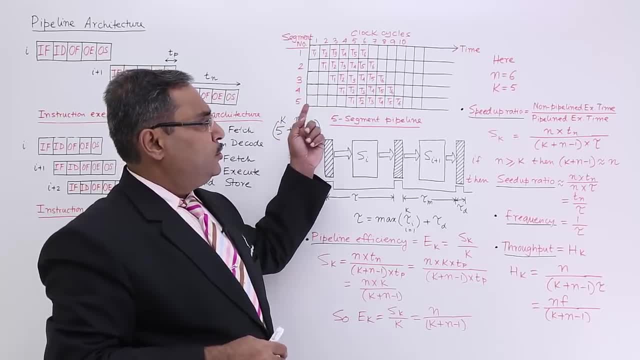 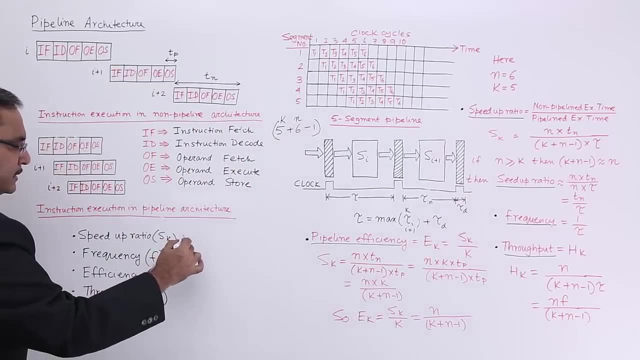 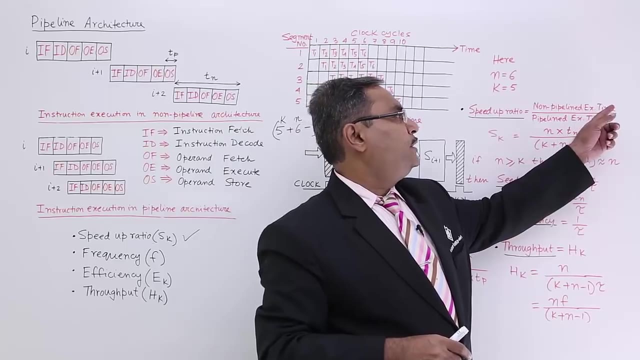 k is equal to five, because i'm having five segments. so this is their case. so now, what is the speedup ratio? so let me discuss the first one. let me discuss the first one: the speed up ratio. what is the speed up ratio? speed up ratio is nothing but non-pipeline execution time by pipe. 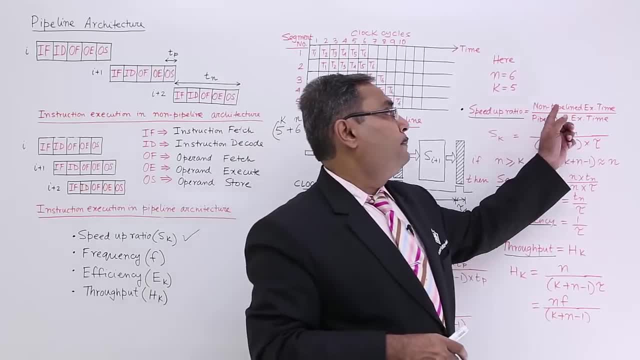 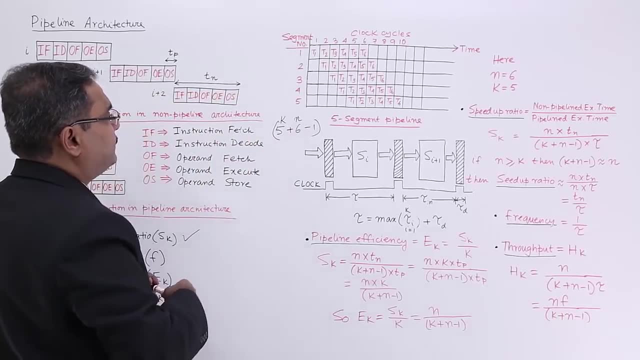 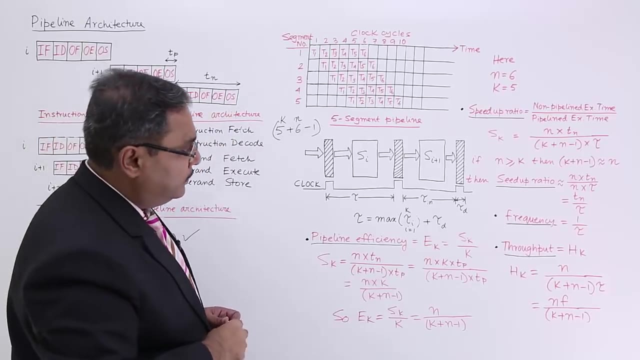 execution time. So speed up ratio is nothing but non-pipeline execution time by pipelined execution time. Now see, let us suppose this is the T n, this is the T n. T n means the total instruction execution time. Now consider this very particular diagram. Here I am having 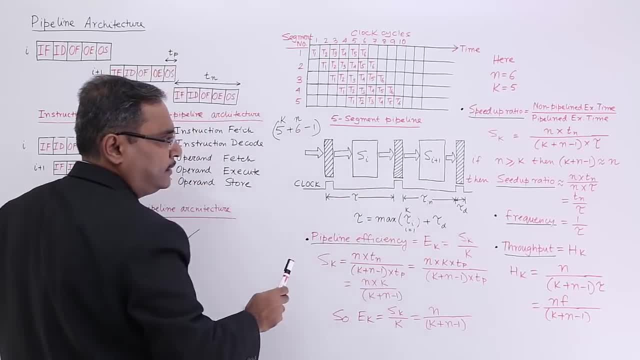 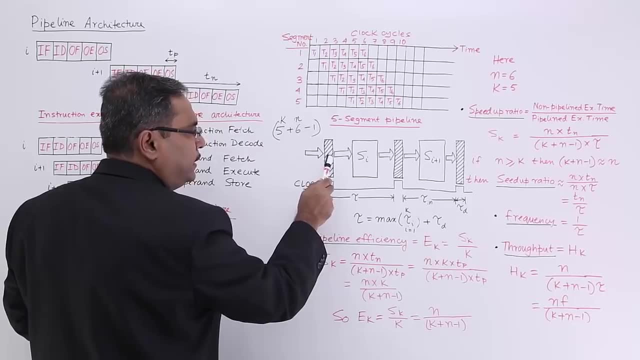 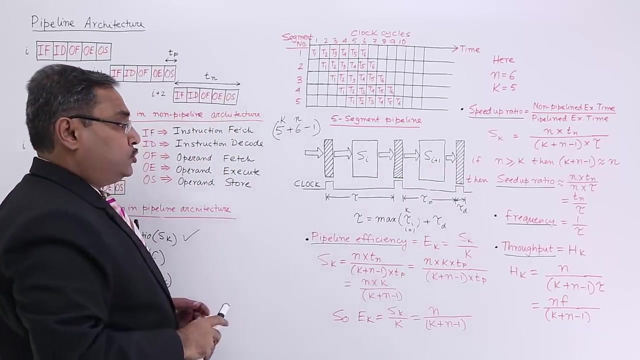 S i th phase and S i plus 1 th phase. In between we are having this latches. When the clock pulse will be falling, then this latch will be enabled. then inputs can go to the output of this latch. Inputs can go to the output of this particular latch. So this is my latch. 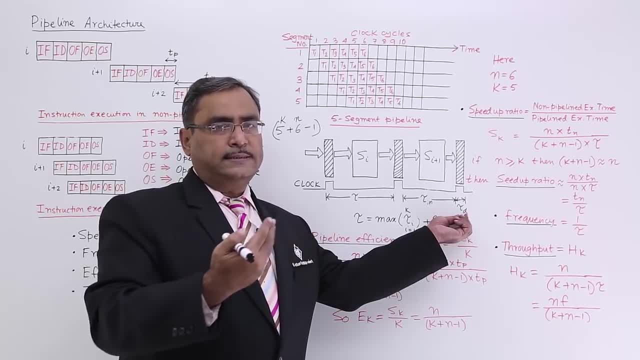 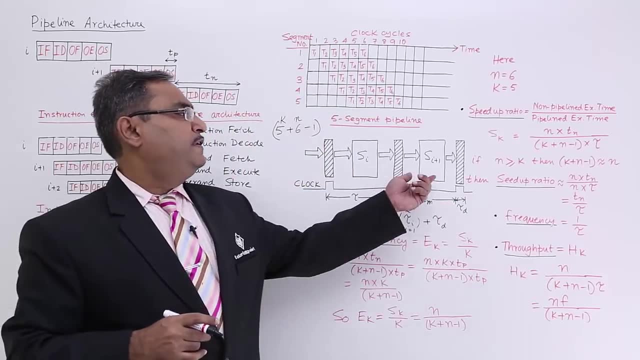 delay. that means input will go to the output, So it will take some time. This is known as latch delay and this is known as the phase duration. This is the phase duration. So output phase, instruction phase, whatever it is. So these are phase durations. T n. 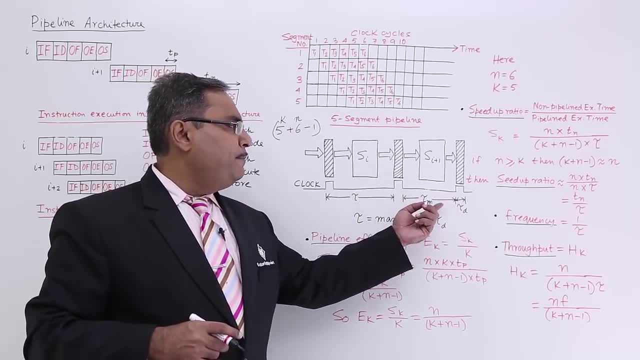 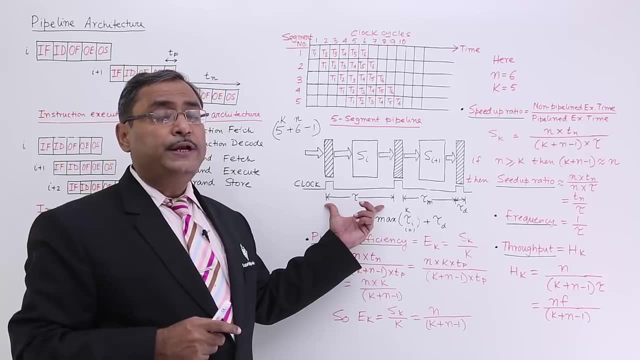 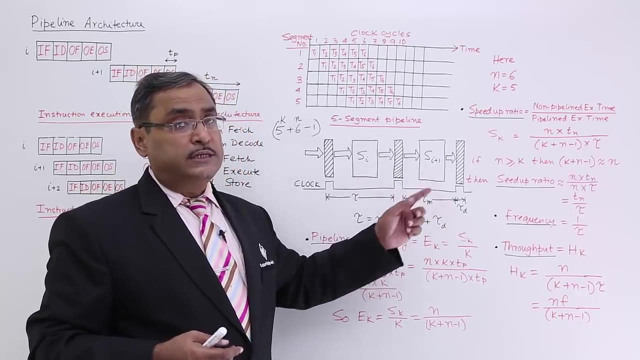 So tau is nothing but T n plus T d. So tau is nothing but T n plus T d. What is tau? Tau is the clock cycle period, So there is a time period of this particular clock, because different phases will have different durations may have. I cannot ensure you that all the 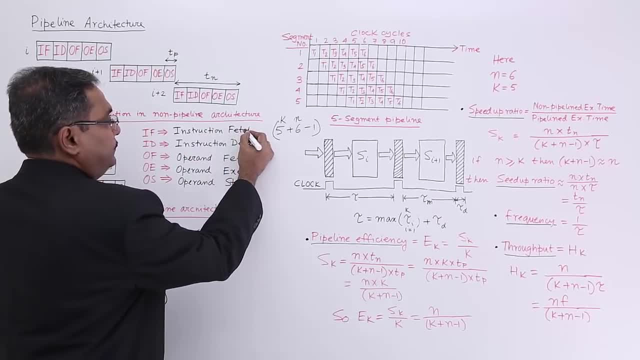 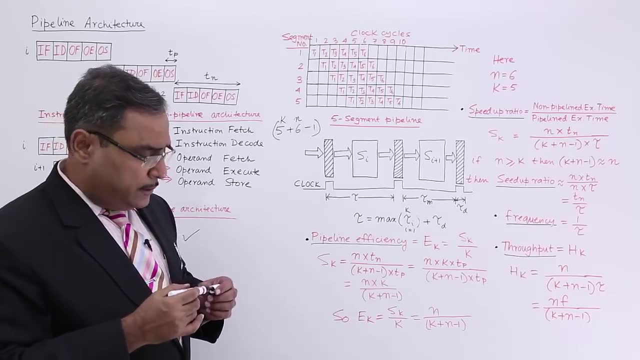 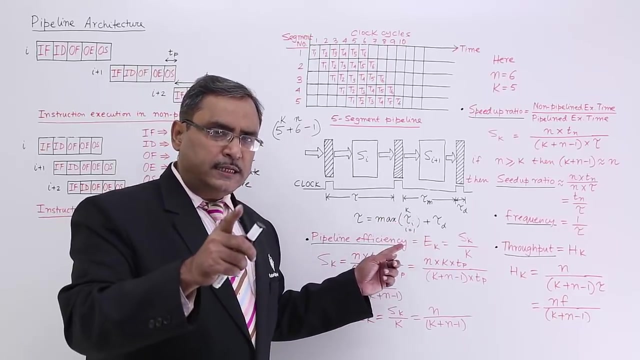 phases will take the same amount of time during the execution. I cannot ensure you that one, because of output phase, may require more time than operand phase might be, or say, operand execute. So that is why it is of a common practice that for all the phases- how many phases are there? K, number of phases. So for all the phases. 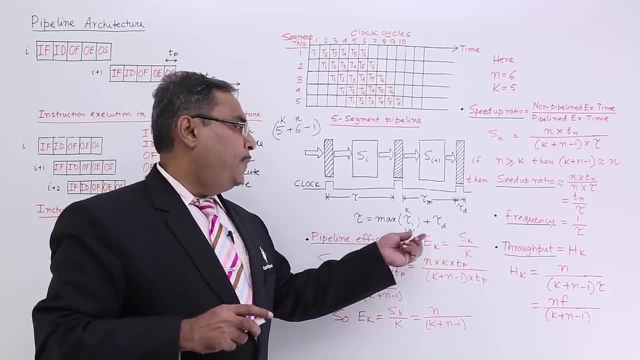 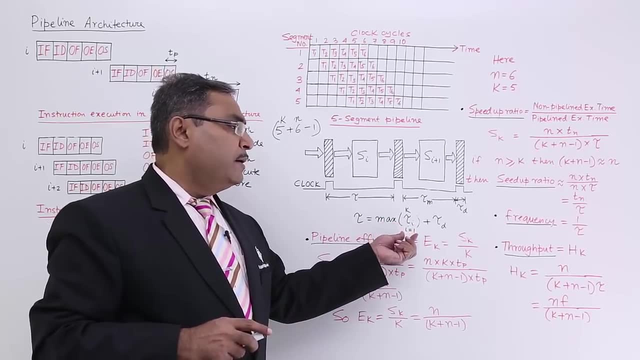 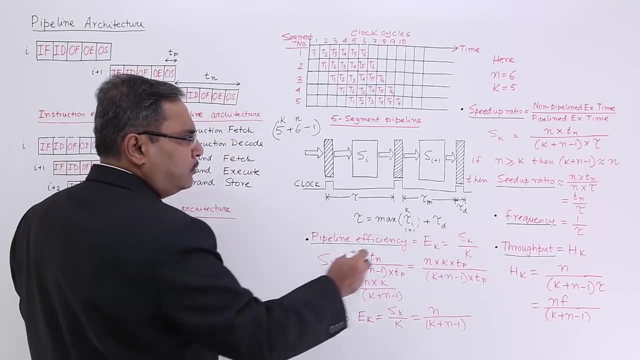 I shall calculate the maximum duration of them plus the latch delay will be the time period. So it is a very famous equation. So that is my maximum phase duration plus latch delay will give you the time period. ok, So now what is the frequency then? 1: 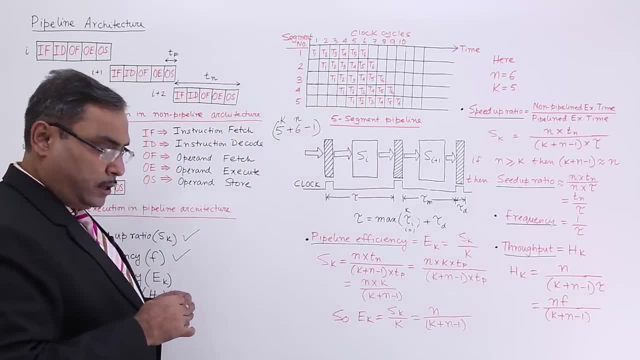 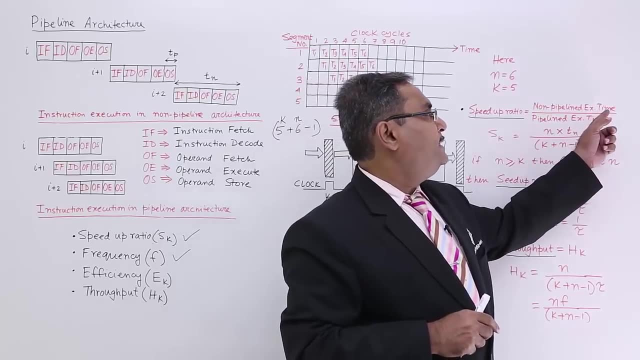 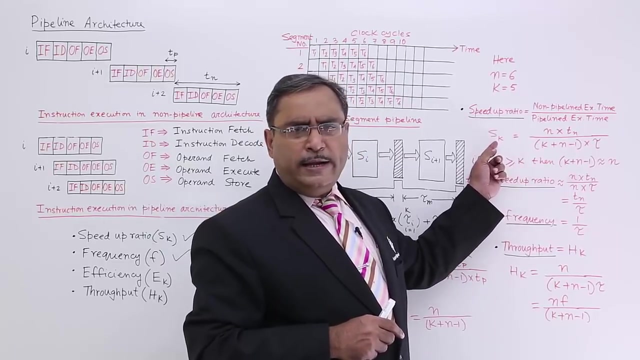 by tau. So what is the frequency? 1 by tau? good, Now please come to the speed up ratio again. Speed up ratio: non-pipeline execution time by pipeline execution time. Speed up ratio s of k is equal to why I am writing k here? because we are having k number of phases. 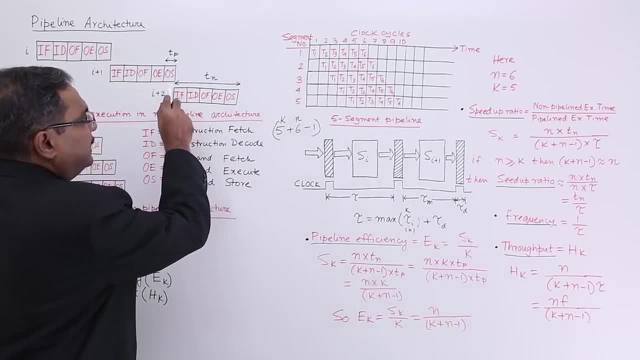 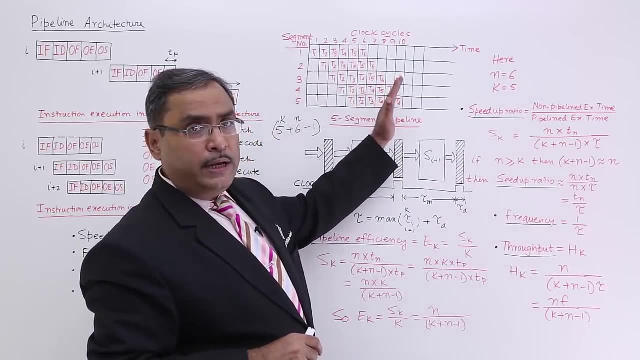 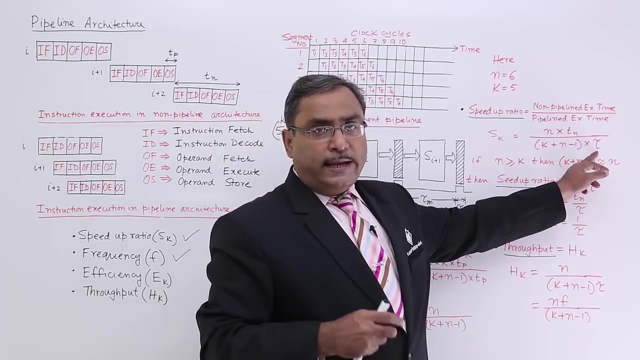 n number of instructions. what is t n, that is the instruction execution time n into t n by how many clock cycles it required, how many k plus n minus 1 number of clock cycles. so into the clock cycle duration. so that is the time period, so that is a tau, so that is. 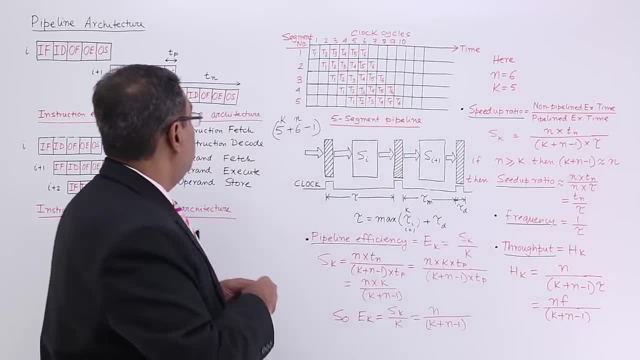 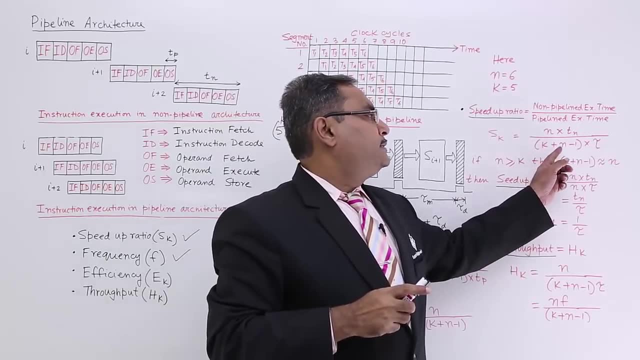 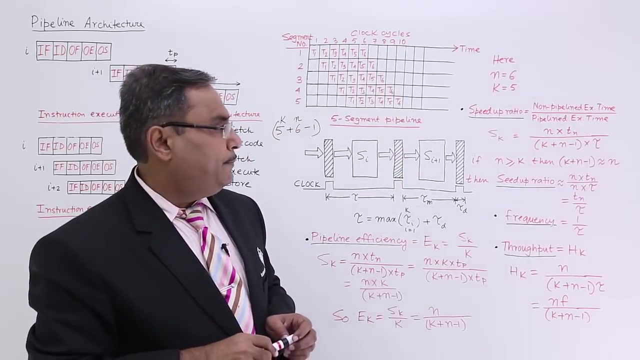 my s of k. so n into t n means this one, this duration for one instruction, for n number of instructions. it will be n into t n, k plus n minus 1 into tau will be the pipeline execution time. so their ratio will give you the speed up ratio time. now, if n is very, very much greater, 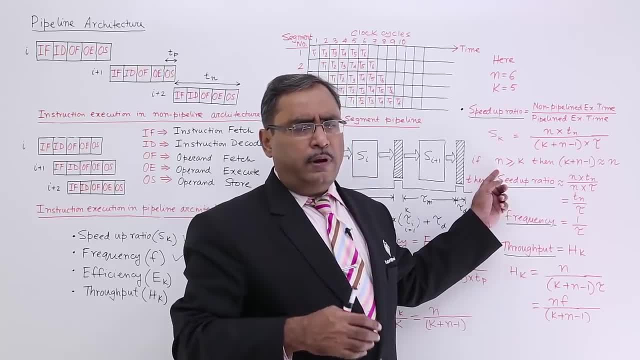 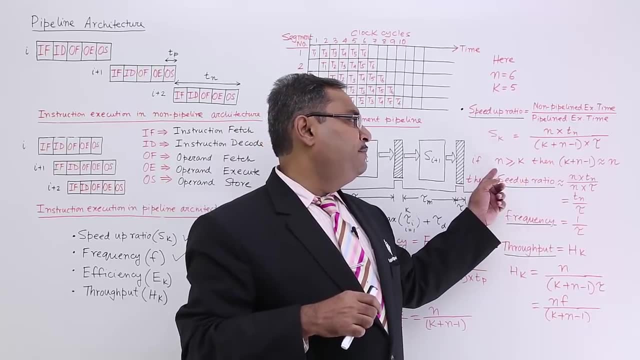 than k. we know that n can be a very large number. large number of instructions are getting executed, but k is fixed for the architecture. so in the case if n is very, very much greater than k, then k plus n minus 1 will be almost equal to 2.. 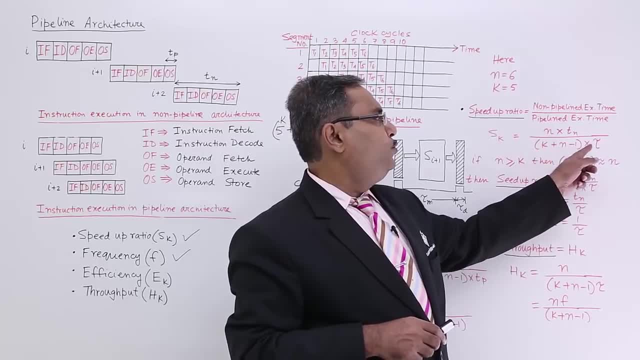 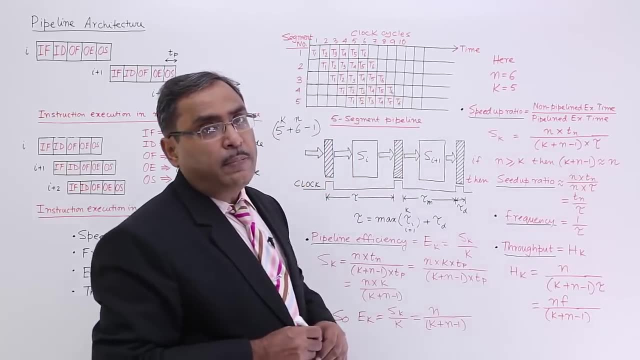 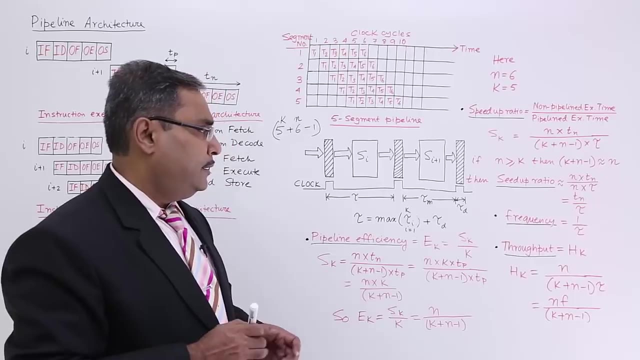 to n. So here we will be getting n into tau, here we will be getting n into T n. So speed up ratio will become almost equal to that is T n by tau. So that is a one assumption assumption I am having that is n is very, very much greater than k. So now I want to calculate. 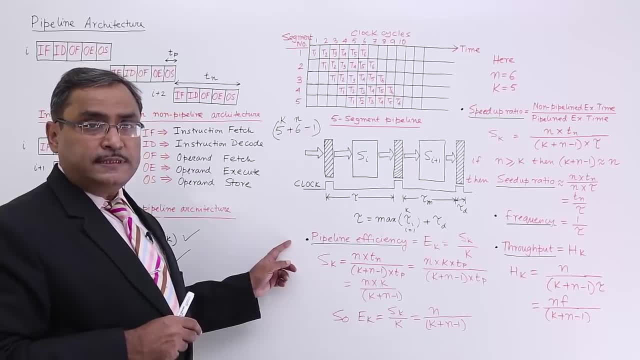 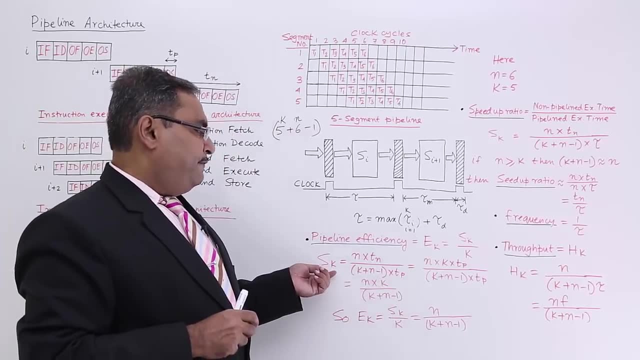 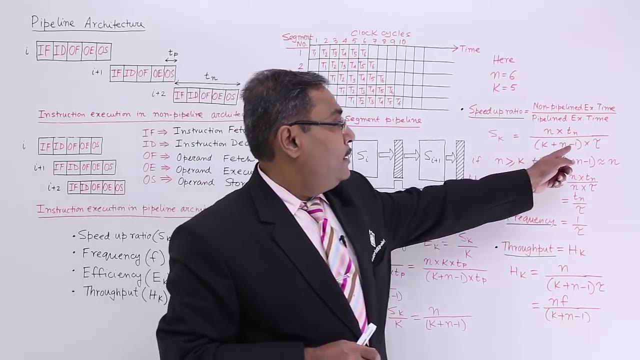 the throughput, then I shall also calculate the efficiency. ok, Let us go for the efficiency at first. Efficiency means we are having this S k: we are having n into T, n by k plus n, k plus n minus 1 into tau. I have written the same. I can also make. 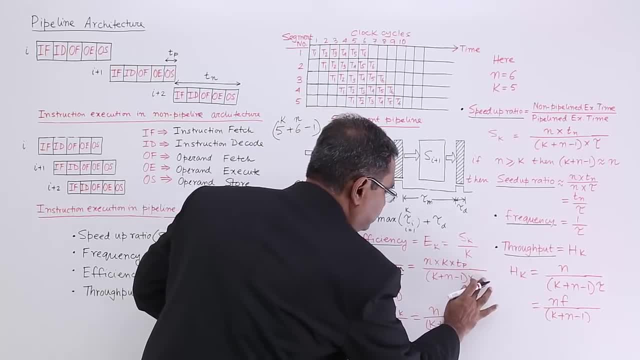 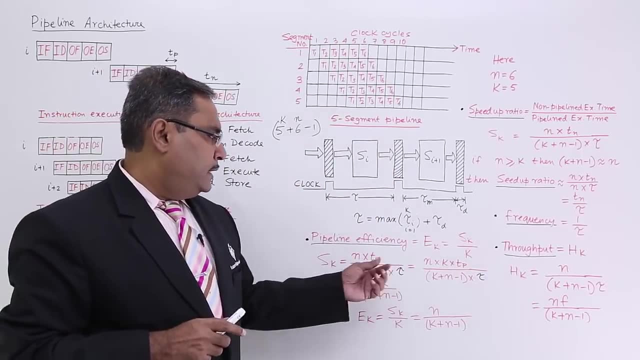 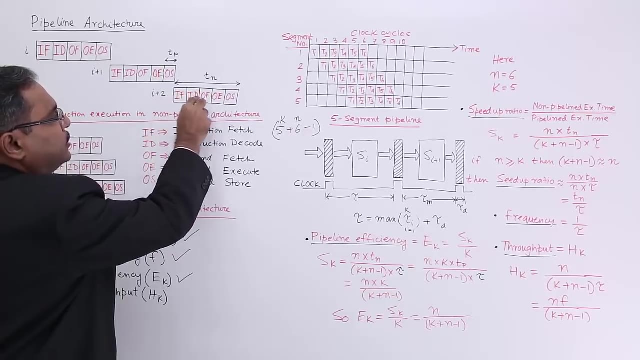 it tau also no issues. So same thing: tau, T p means phase deviation. So here the phase deviation is tau. So now what is happening? you see, T n means what means T? n means k into T p, T p means the phase duration, So k into T p. So that is. 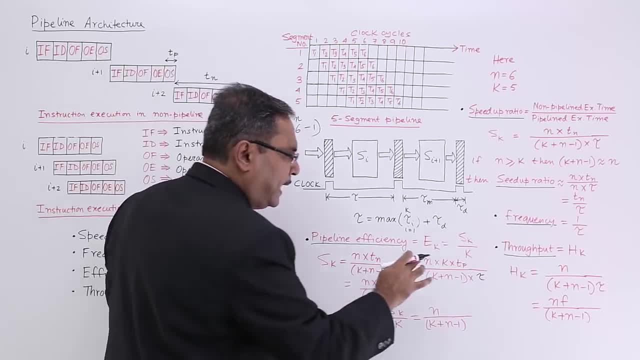 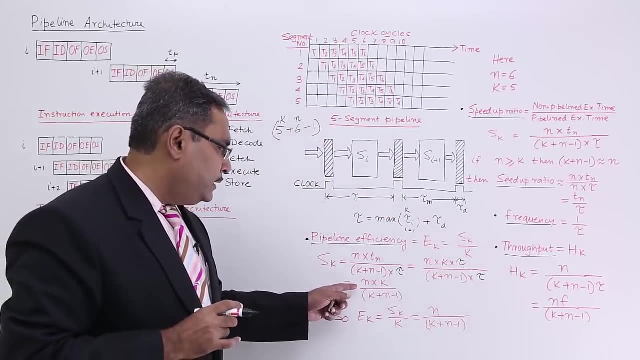 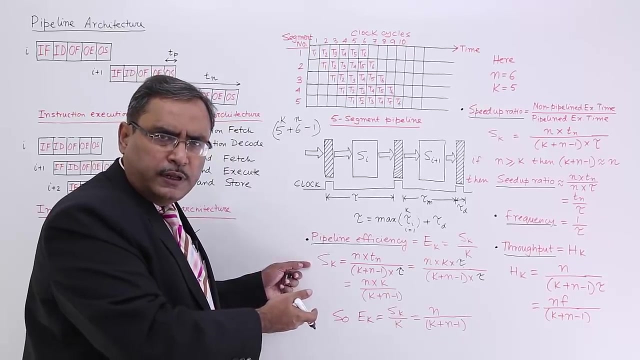 the, that is the k into T p. we are having this one, So T p can be also written as tau, because already we have discussed tau here. So if you go on dividing, so ultimately you are remaining with n into k by k plus n minus 1.. So that is my another expression of this. 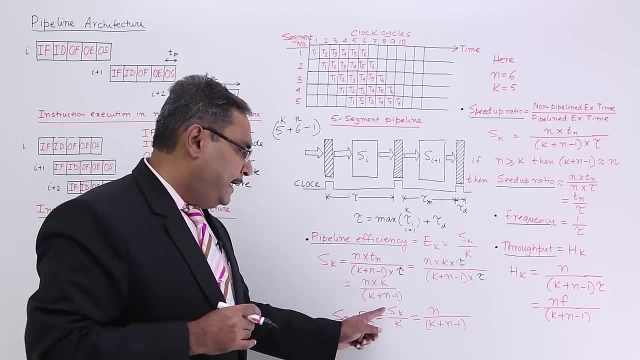 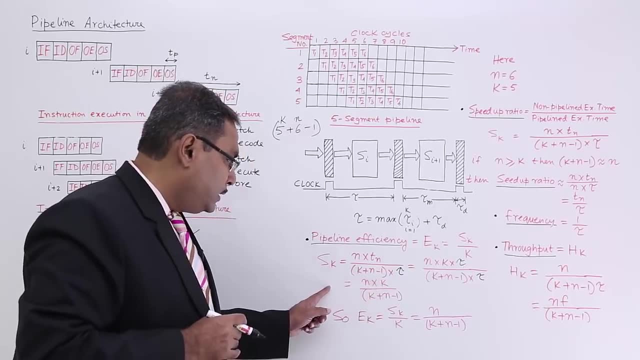 s of k. Now, efficiency means x k by k, x k by k. So s k is there, k is there in the numerator, So it will come down to the denominator. So it will be n by k plus n minus 1. So 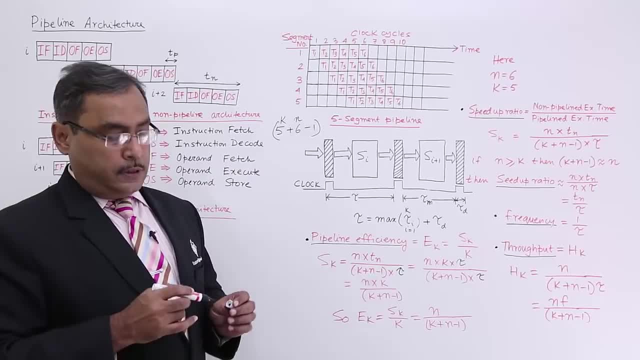 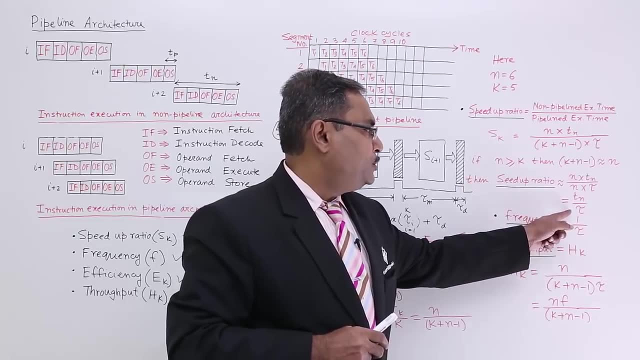 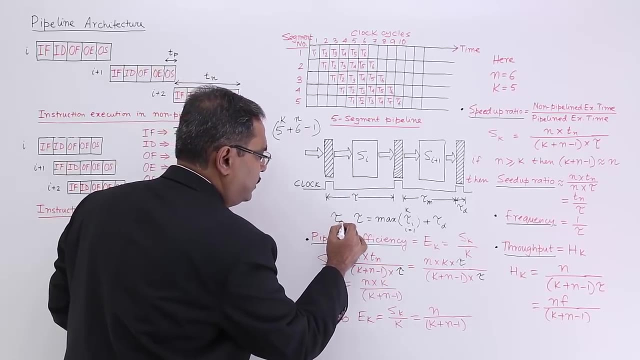 that is the expression for the efficiency of the pipeline. So speed up ratio. I have done the calculations- one assumptions, So speed up ratio has become this one. So here the phase duration is Almost equal to. there is a phase duration is equal to the time period which is max of 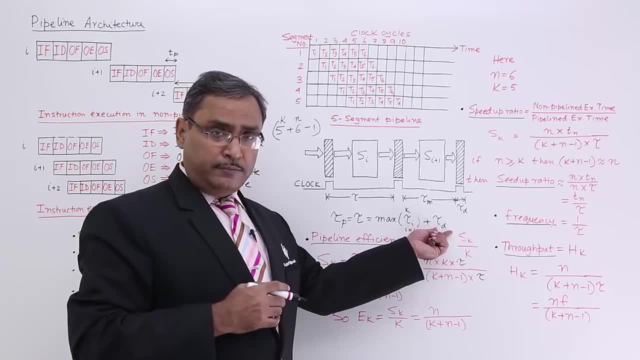 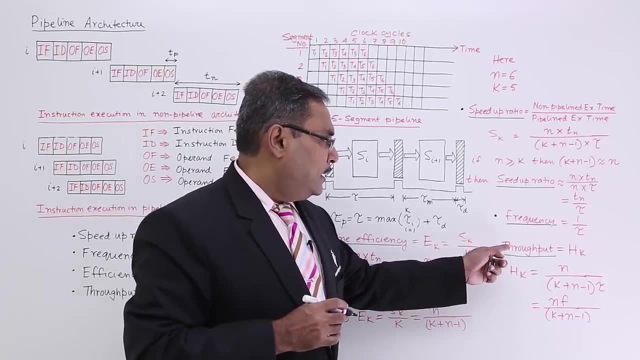 the phase durations plus the latch delay. I told you this one from this diagram. It is there also mentioned, and then we will be having this frequency. I have discussed, So last topic is my throughput. So last topic is my throughput, So let me discuss the throughput. 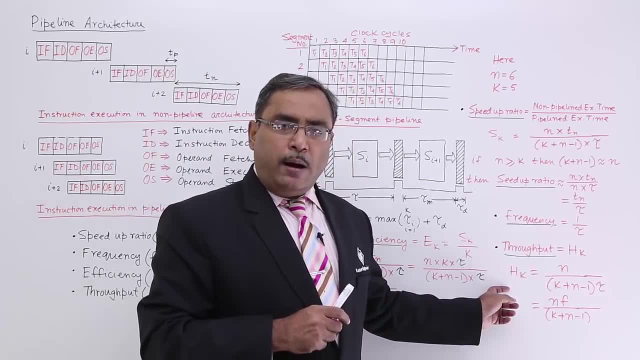 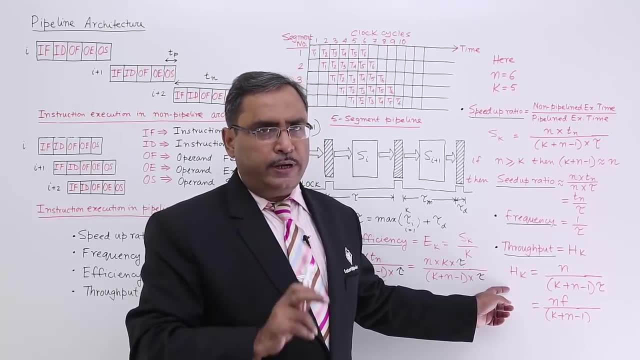 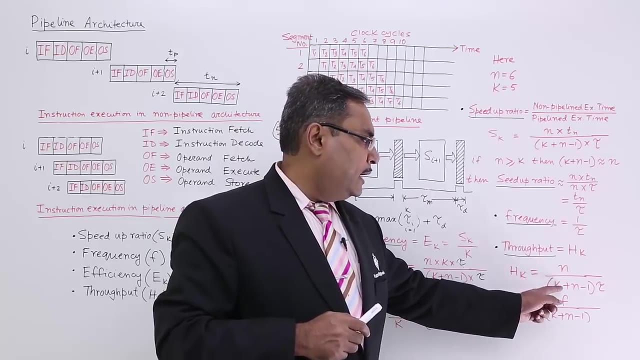 here. So what is the throughput? Throughput means number of instructions executed per unit time. Please listen to me. Number of instructions executed per unit time. How many instructions have got executed? N number of. What is the total duration? k plus n minus 1 into tau, So there is a. 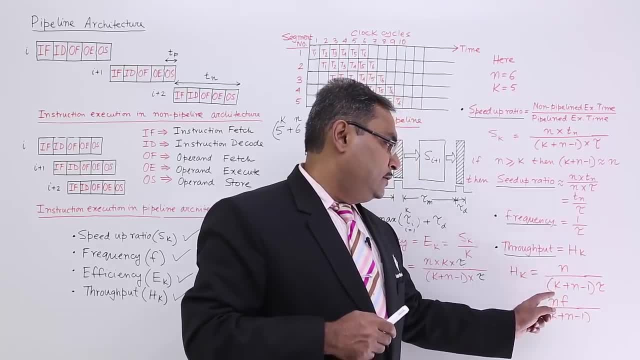 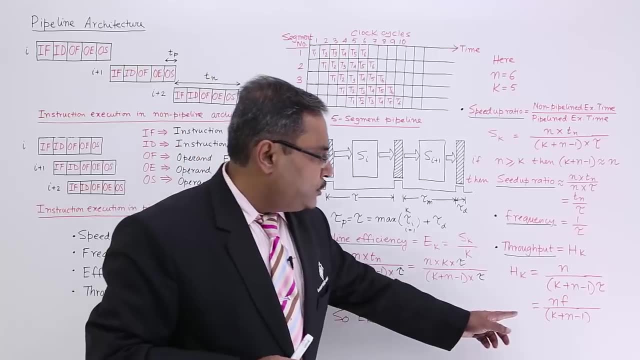 total duration, So n by this, n by this, will be the number of instructions executed per unit time, and that is known as the h of k. So h of k will have the formula like this, and it is quite obvious that frequency f is equal to 1 by: 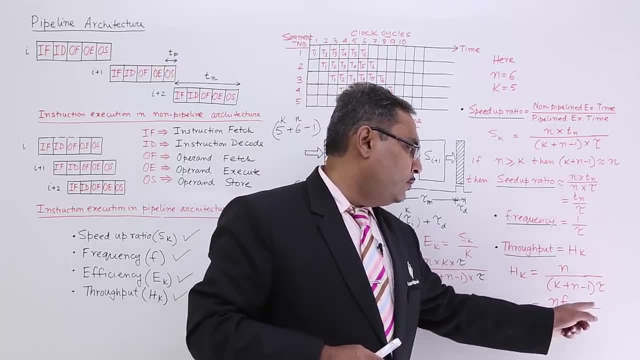 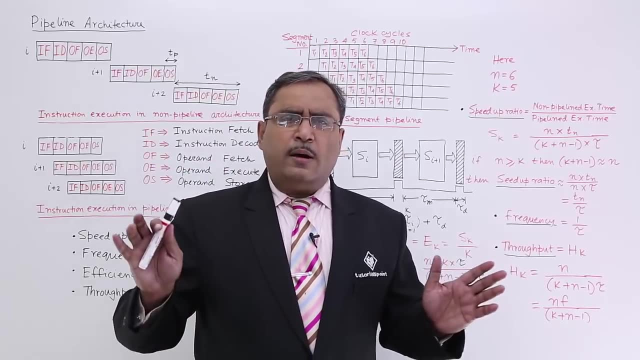 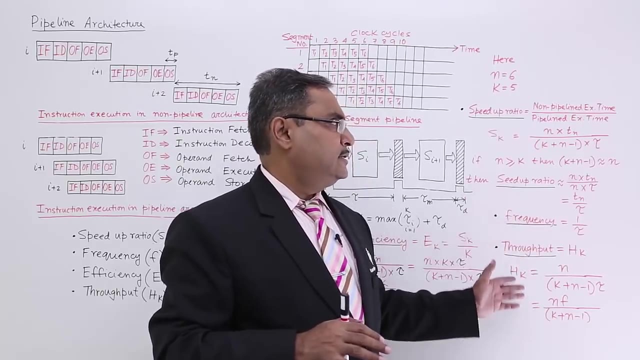 tau is equal to 1 by f. So this 1 by tau can be also replaced by f only, So n into f by k plus n minus 1.. Several number of numerical problems may come on this, on these particular formula. Please remember them. and the deductions derivations are quite simple. So there is: